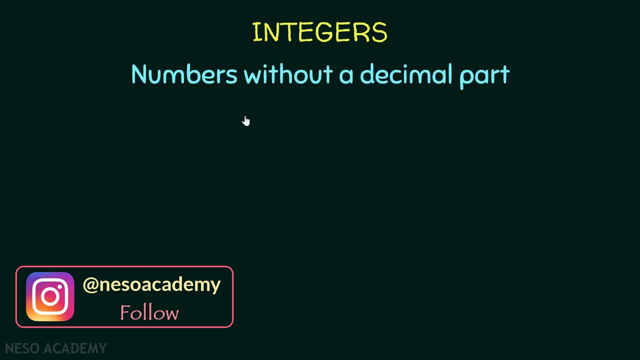 What are integers? An integer is a number without a decimal part. So here are some examples: 1, 2, 100, minus 4, minus 9, 0.. All these are examples of integers. They are numbers without a decimal. 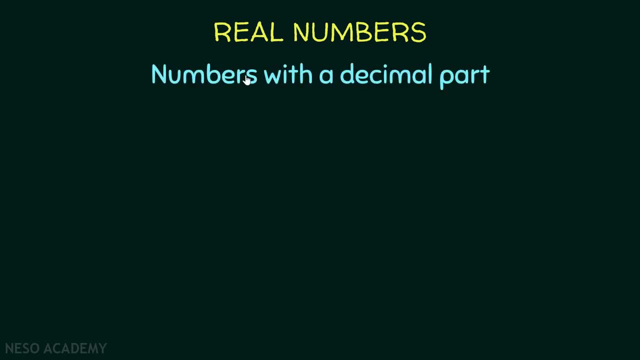 part. Alright, Now let's see real numbers. So they are numbers with a decimal part. Here are some examples. As you can see, all these numbers have a decimal part, Even 1.0 and 0.0.. They are. 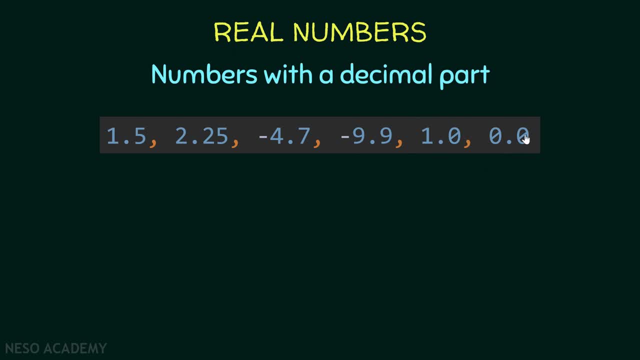 considered real numbers, Alright. So we can conclude that an integer can be a real number. So if you have a look at these numbers, they are considered real numbers, Alright. So if you have a look at these numbers, they are considered real numbers, Alright. So if you have a look at these numbers, 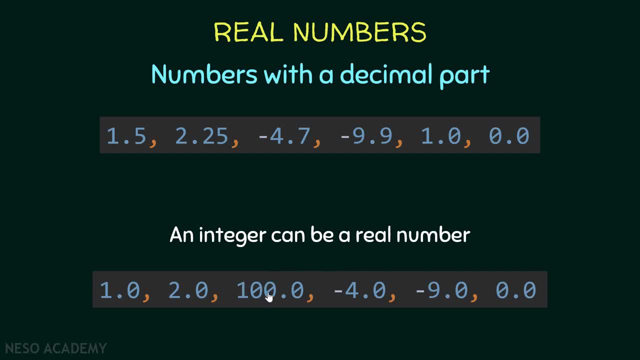 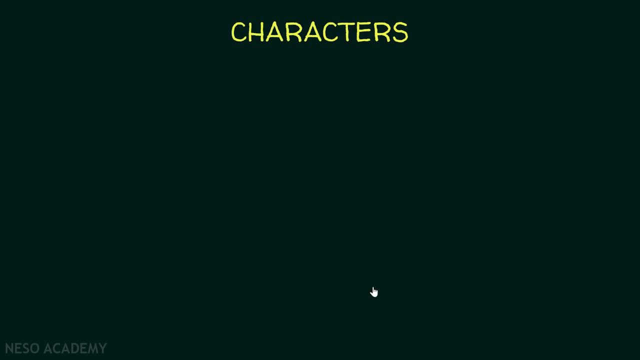 they are considered real numbers, Alright. So if you have a look at these numbers, they are considered real numbers. For example, if we have 100, if we simply add 0.0, this will be a real number, Alright, And it will not be an integer anymore, Alright, Now let's talk about characters. 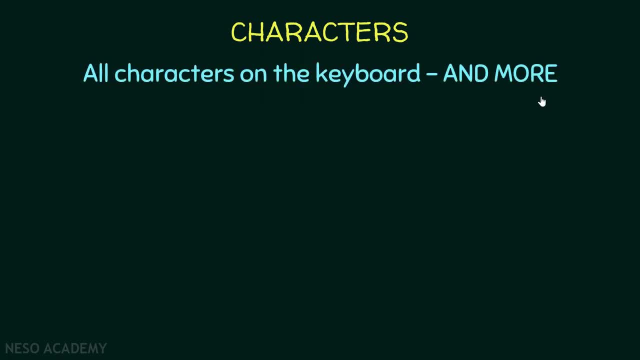 So characters are all the characters on the keyboard and more, Alright. So here are some examples. All these are characters And you can't find all of these on the keyboard Right. So all you have to do is to write a character and put it between single quotes. So, for example, we are putting 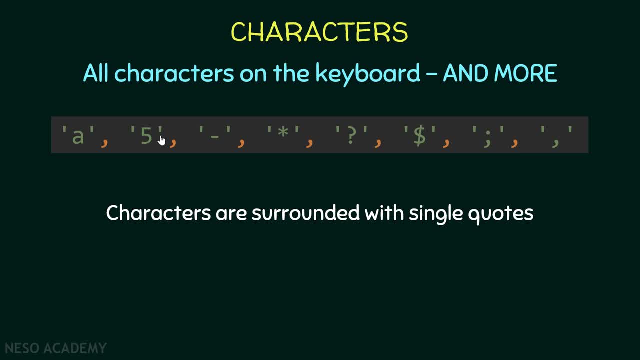 the number 5 between single quotes. So now it is a character, But if you put it inside double quotes it will be a string, Alright. So characters are different than strings, Okay, So also we have the minus sign, the asterisk, the question mark, the dollar sign, the semicolon and even the comma. So 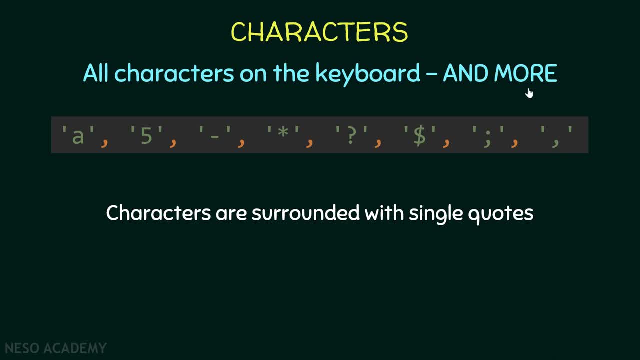 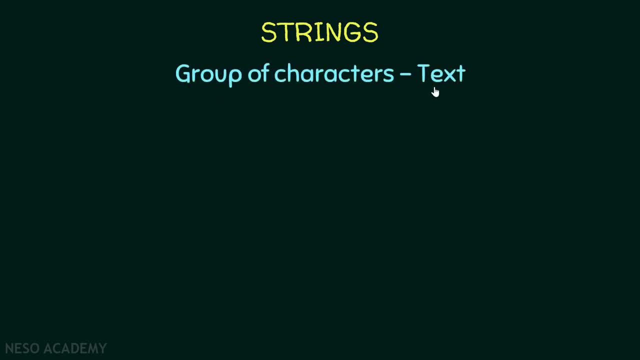 everything on the keyboard can be a character, And we have more, And we will talk about this later. Now let's talk about strings. As you already know, a string is a group of characters or it is a text. Right, So here is a string. As you already know, a string is a group of characters or it is a text. 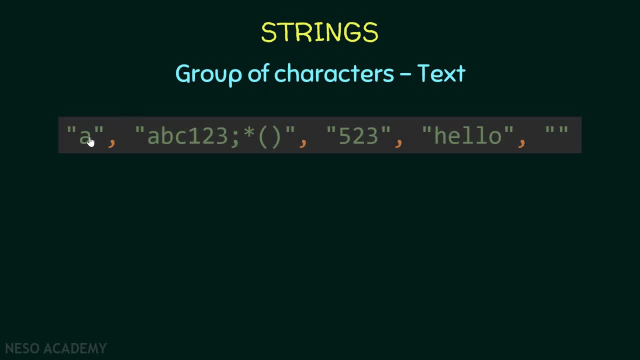 So here are some examples, And you are already familiar with strings. All I want you to remember is that we have a special string, which is an empty string, which contains nothing. Alright, And as you know, we use double quotes when we work with strings. Now let's talk about booleans. 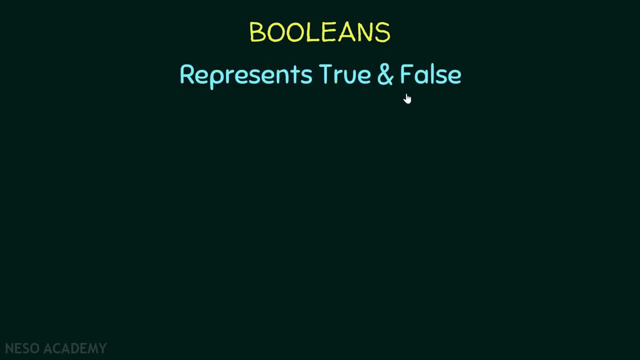 A boolean is a value that represents true and false- Only two values. Okay, So inside Java we can write the keyword true and the keyword false. Now you might ask: why do we need true and false in programming? Well, the answer is simple: We can write the keyword true and the keyword false.